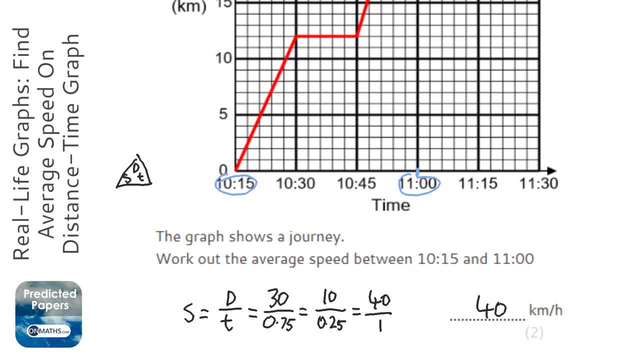 Which is just 40. Or you can do it 30 divided by 3 quarters. So 30 divided by 3 quarters, Which is the same thing as there, And then you do same change, flip Or KFC, Change that to a times and there should be a 4 at the bottom there. I don't know why I've written a 7. And flip the second one. So 30 times 4 is 120, divided by 3 is 40.. Loads of different ways of doing that without a calculator. Obviously, we've got a calculator type. Type in 30, divided by 0.75.. 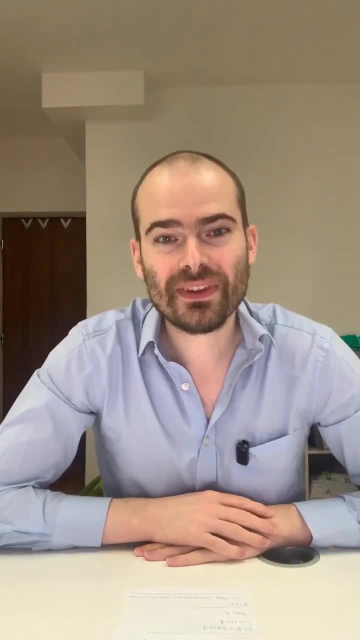 Hey guys, if you are applying for a Czech visa or a residence permit, or you're extending it, or you're bringing your family coming here as a student, whatever- you will at some point need to prove that you have a health insurance. And since the monopoly in the health insurance 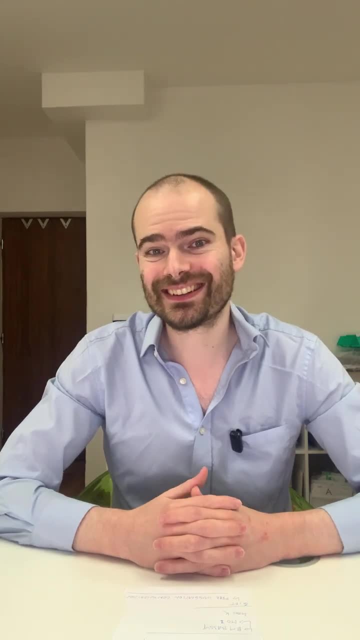 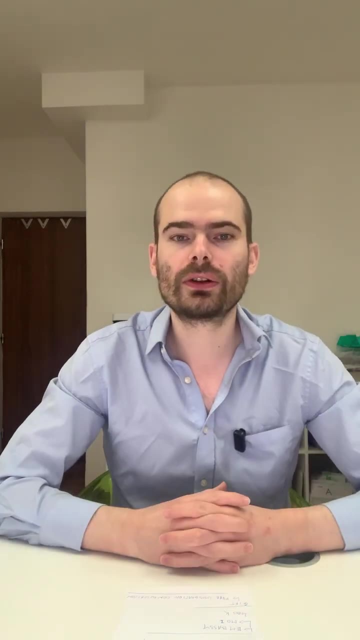 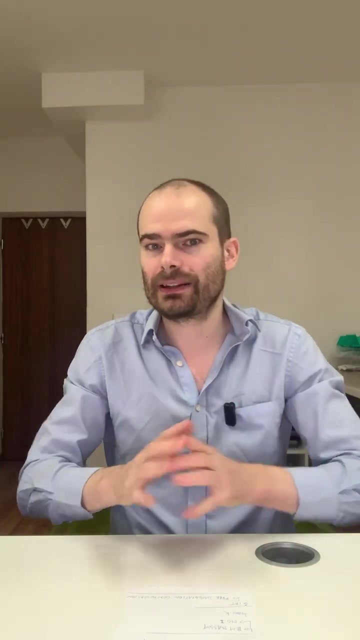 in the private health insurance in the Czech Republic has been cancelled since September 2023,. there are plenty of updates and plenty of news which I wanted to share with you, And I will also have a special gift for you. So stay with me until the end. It will be like. 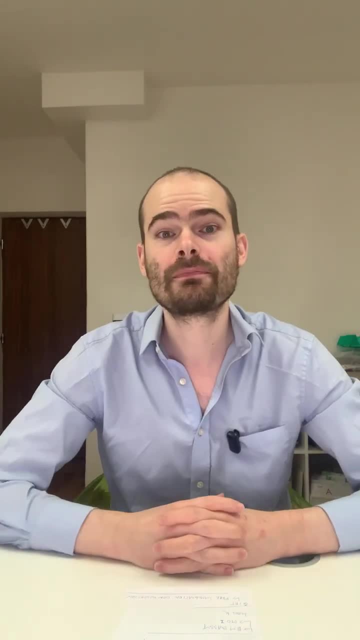 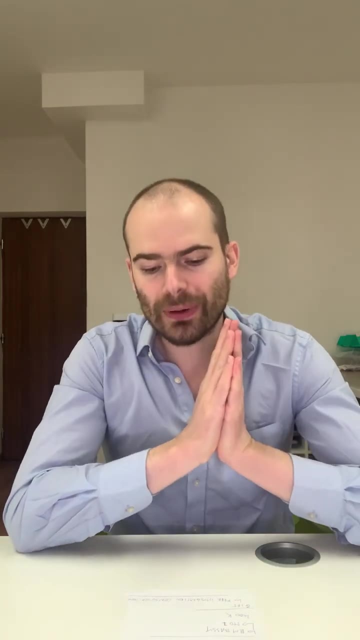 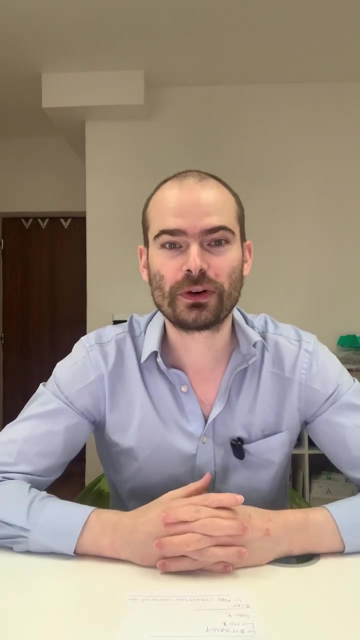 five, six minute long video. So stay with me and you'll get all the information plus an extra gift for you. So a couple updates, a couple confusions that are there and then the special gift That's the structure of the, of the live stream or the video. So, first of all, since the monopoly was cancelled, there are seven different companies offering health insurance- private health insurance- in the Czech Republic. We work with six of them, So we have like a pretty big range of the insurance we can offer you. So if you want to get the best quotes, get in touch, because we've done a lot of. 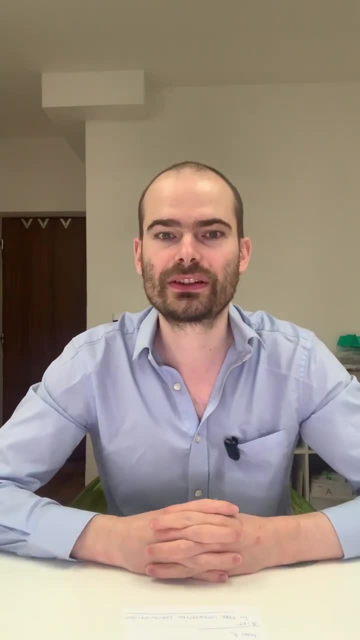 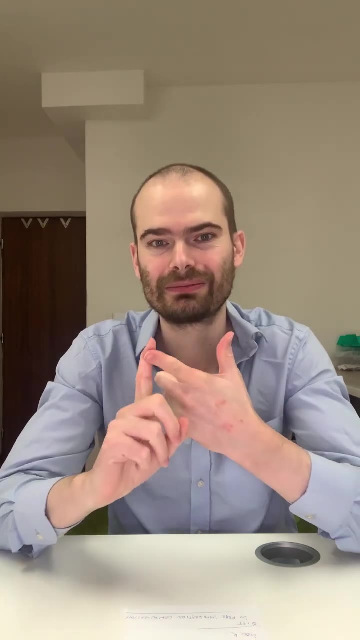 insurance for insurance companies. So we have the best quotes. We have the best prices you can get on the market. So if you need a quotation, send us a date of birth, ideally the type of visa you're applying for or you're getting, or why do you need the. 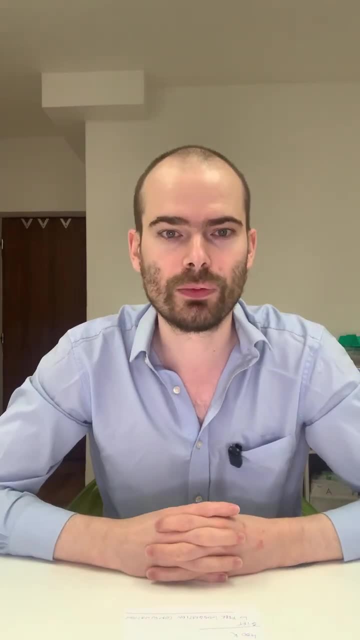 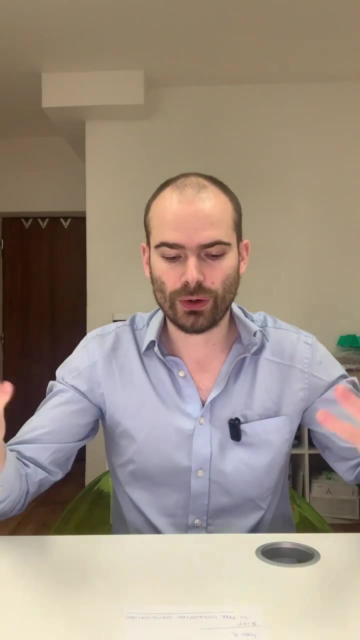 insurance for for how long, and then we'll be happy to send you a couple quotes with the different prices: different options, different coverages, different different companies. Yeah, So that's the price. Obviously, I cannot share the price directly in the live stream because about If, if clients actually are getting the insurance for the price, if there is some room for increasing the prices or if they have to decrease. So they've already changed the prices a couple times, Yeah, And that will be happening consistently. So at least for the next couple months, then it will probably